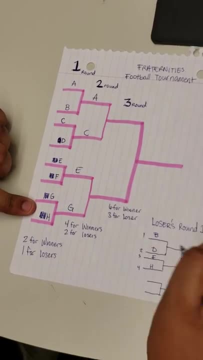 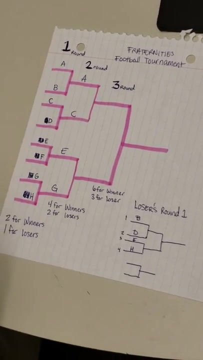 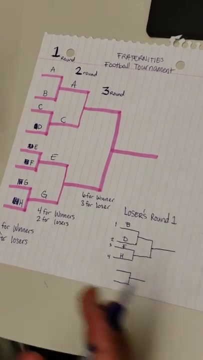 F will go to the loser's bracket And H will go to the loser's bracket. Now, in the losing round, teams will play one more, not a full game. they'll basically play to see who gets the first touchdown, after which they'll be placed. 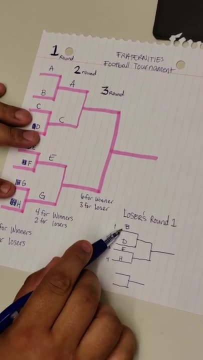 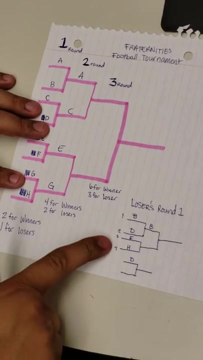 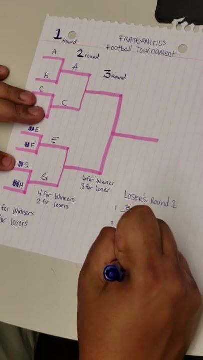 accordingly. So if B scores the touchdown against D, B will move on. D will go down to another game to wait to see who beats, who wins out of F and H. So let's say F beats H. H comes down here Now. 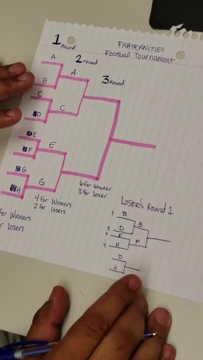 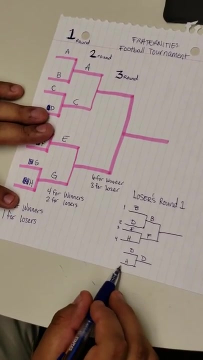 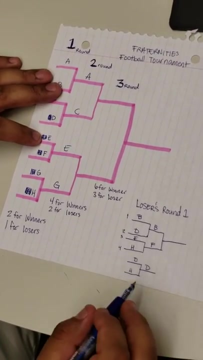 D and H will both be competing for a certain number of points too. So say D beats H, That means H is the ultimate loser. They received one point in the round that they actually competed in, and they received one more for this little mini tournament, So they'll have two points total. 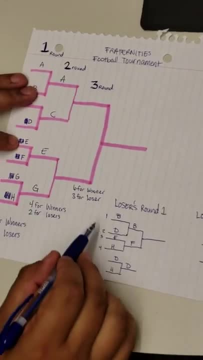 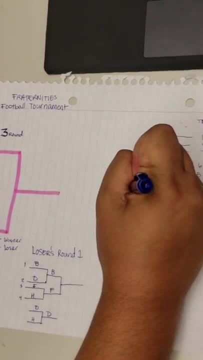 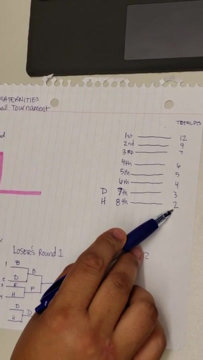 So I'll put them over here. at eighth place, D lost in the mini tournament but won ultimately against H, So they'll get two points to be placed right here on seventh. So they're one. if you look at it, they get one point for participating in round one. 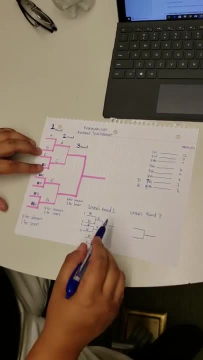 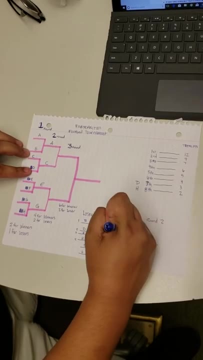 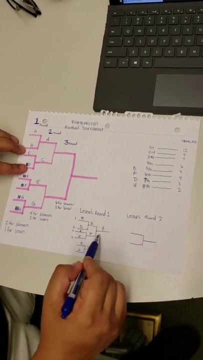 and then an additional point for getting their placement in the mini tournament. So out of the four, fourth, third, second and first, which we'll decide right now, let's say B beats F, So the first in the loser's tournament will get another additional four points. 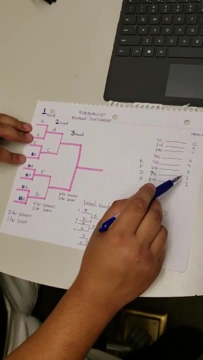 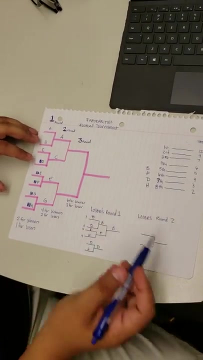 plus their one for participating. So they'll start with five And then it goes all the way down. Now they can't earn any more points for football. They just have to look forward to the next couple of events. Let's go back to the winning rounds. So here A is going to beat C. 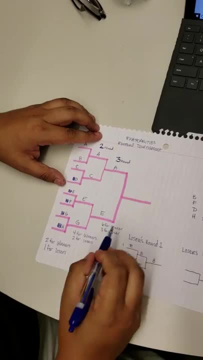 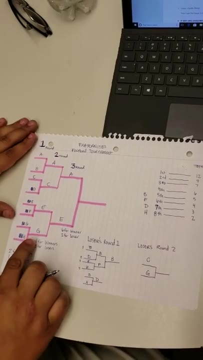 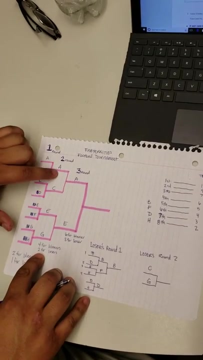 and E is going to beat G Now. that sends C and G down to the loser's round two. Now they've already earned- all of these teams have earned- two points for winning round one, and then they will receive two points for losing round two. 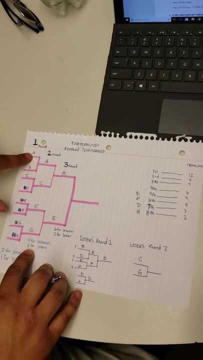 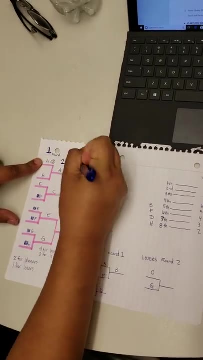 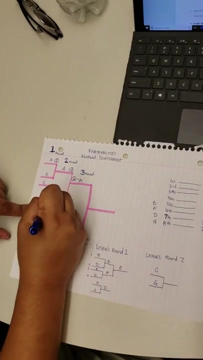 Winners of round two receive four points. So that means going from round one, two and all the way to three. A has two points for winning here. four points for winning here mean going into round three. they have six points. Same thing with E: two points for winning here. four points for winning here. 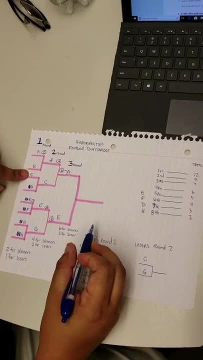 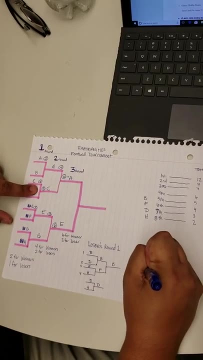 six points total in the championship round. C has two points for winning here and only two points for losing here, giving them four points total. So I'm going to go over here, write four, And same thing with G: two points for winning the first round. 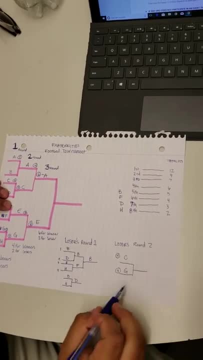 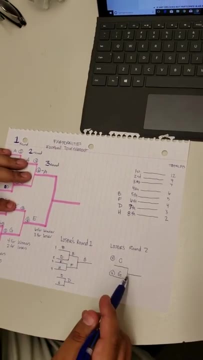 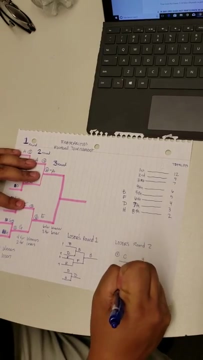 two points for losing the second round, for a total of four here. Now, obviously, they're not going to be lower end points than the teams that lost in the first round, So whoever wins out of these two will receive an additional three points with the loser. because they lost in the second round to go to round two, will receive two points participation If they lose here, and that's going to be another, whoever scores a touchdown first. So if G loses, so G loses, so they have their four plus two gives them six. 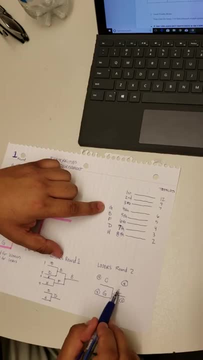 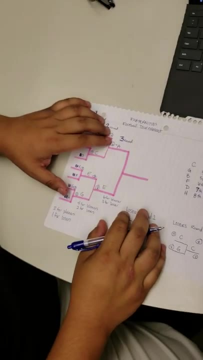 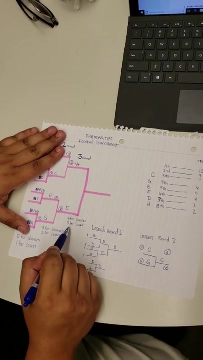 That's where the six comes from. C wins: they have their four plus the three puts them in. third gives them seven. Now you have A versus E in round three. The winner of the championship round will receive six points. The loser will receive three. 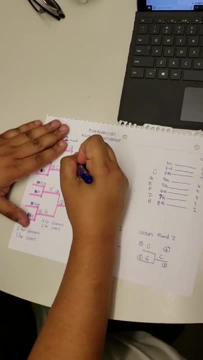 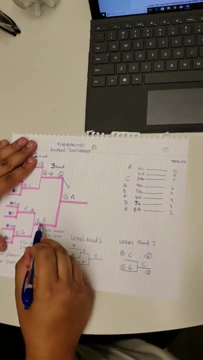 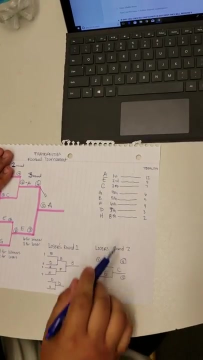 A is going to take it all the way to get their six, plus an additional six, for a total of 12.. And that's why they'll go here. E will get their six, plus losing points of three to get nine, And that's how the tournament breaks down. 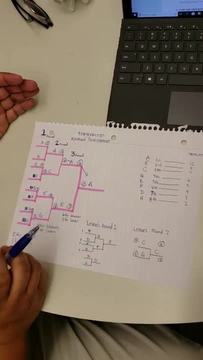 If you have any other questions or need this explained to you in person, please either contact myself or Gilbert.